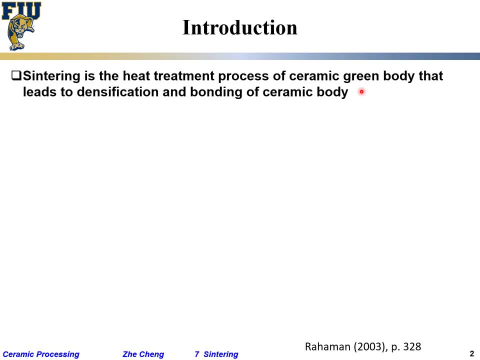 to high enough temperature, which is not difficult to reach, and then everything become together, bonded together, liquid, right, they bond together everything together and then, when they solidify, typically doesn't have too much porosity, unless my process is poorly controlled. 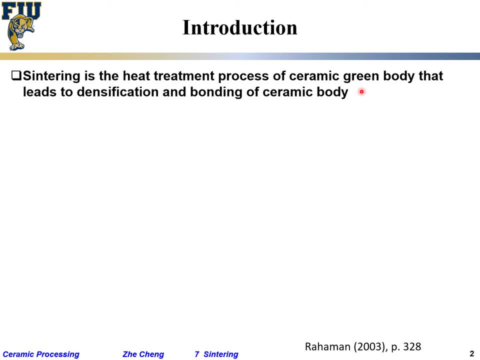 makes sense. so for metal people don't use sintering that often. of course there's some type people call powder metallurgy. people sinter some metal, for example tungsten. you sinter them. you don't really go to the tungsten melting temperature 3000 something. 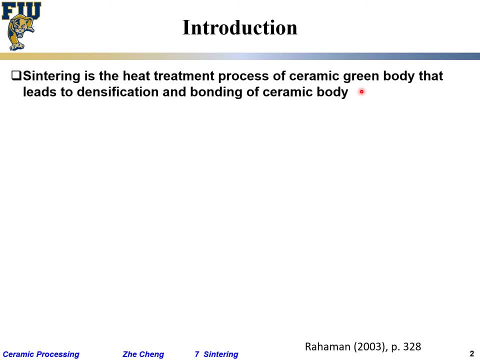 to melt it and then get solidified tungsten, the reason being tungsten to get 3000, the thing difficulty would be what mold I'm going to use to hold my 3000 above degree C liquid tungsten. I have no mold, unlike for aluminum, for copper, even for steel. I can just. 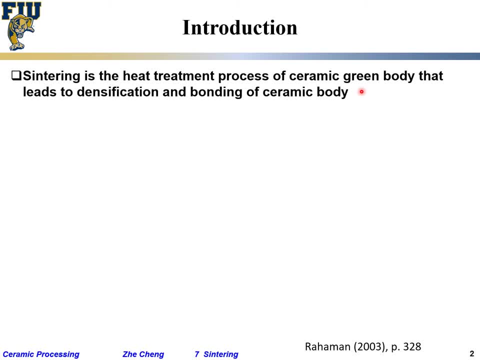 use sand or some other ceramic as my mold. but for tungsten, what am I going to use as my mold? I don't have many good choices. you see the point. that's why sintering is primarily for high temperature. we said most, not most, but at least a significant portion of ceramics, those oxides, 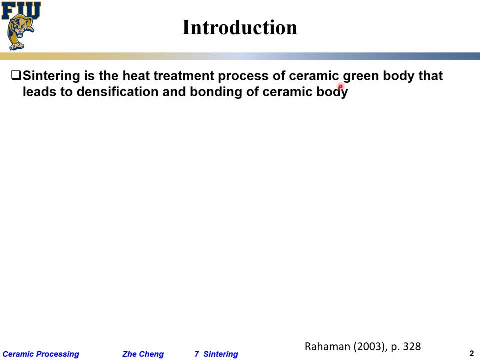 those carbides, borides, nitrites, quite often have very high melting temperature, which means it's difficult for me to melt it and densify it. so that's why we have to start with so-called powder compact, or we call green body. apply heat but not. 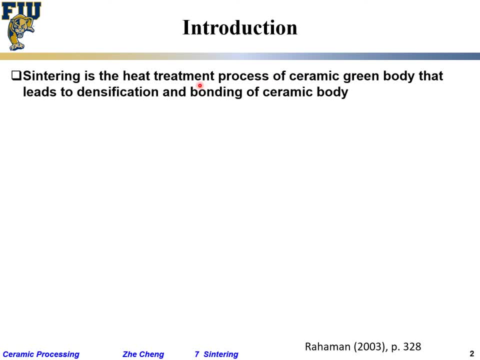 too much heat, not to the point that I melt it and under that condition I remove the pore, which we call densification, and bond the powder together. that's called sintering. okay, there's several major factors that impact sintering. composition right. 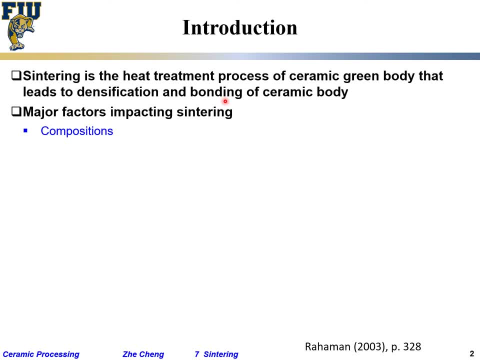 what material are we sintering? I'm sintering aluminum oxide versus silicon dioxide versus carbide versus boride, and even for the same aluminum oxide, I can add different so-called additives, composition- okay, starting powder, characteristics and packing, for example. 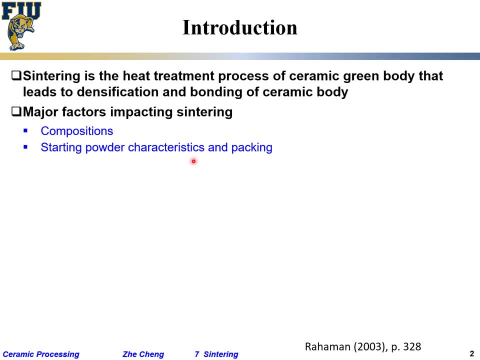 are you using one micron particles or, let's say, 10 micron particles packing? are they more uniformly packed or are they have so-called heterogeneity in between them make sense? are they packed relatively denser or are they packed relatively looser? processing: 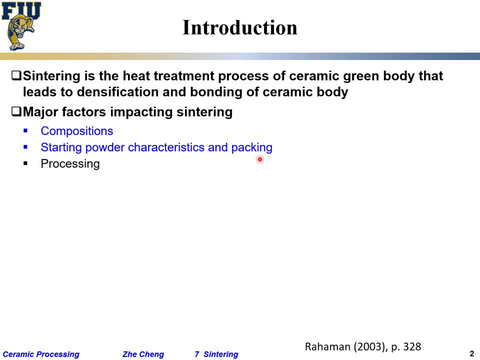 which is: how do you do to the powder compact process? heat schedule: it's always required. you are going to do heat treatment, you are doing sintering heat treatment. you always need to apply heat. without heat the powder does not come together. okay, atmosphere, it's important for 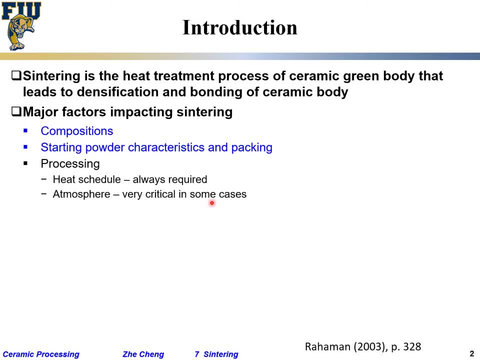 some cases and the reason the cheapest atmosphere we can use, yes, open air, sintering in open air. for most oxides we can do sintering in open air, but if you are doing carbide or boride or nitride, 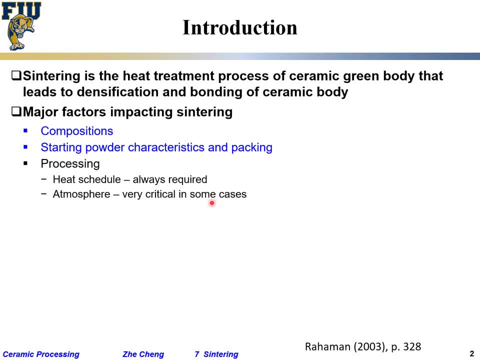 you try to avoid air because otherwise your powder start to oxidize. make sense. and for non-oxide ceramics- that's what we said- carbide boride nitride- you have to use atmosphere, certain inert argon, helium, something like that. okay, for oxides, certain oxides you also have to be. 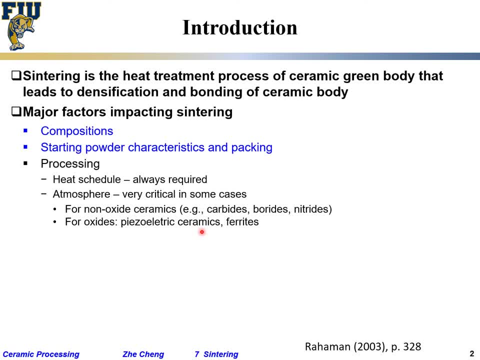 careful with the atmosphere because there are certain oxides that are not exactly stable. there are oxides that when you heat it starts to decompose. for those you have to be careful and to control atmosphere. for example, so-called ferrite or piezoelectric, those that contain lead. 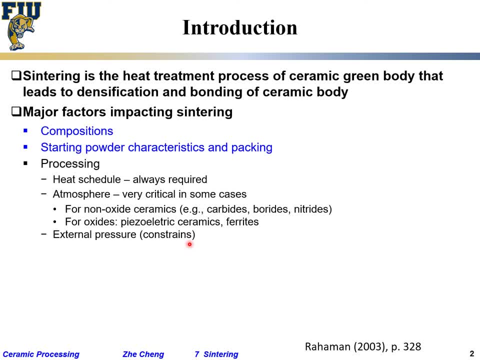 and other components, external pressure or constraints. sometimes people apply it during sintering, for example, so-called hot pressing- hot pressing, which means you are heated up. at the same time you are pressing hot, pressing right, so you may apply pressure during sintering. with that, you may apply pressure to get a green pellet.